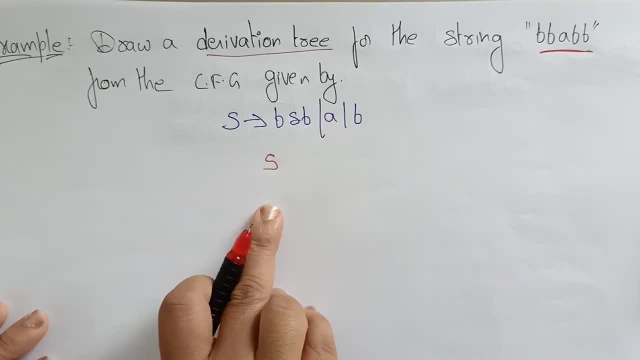 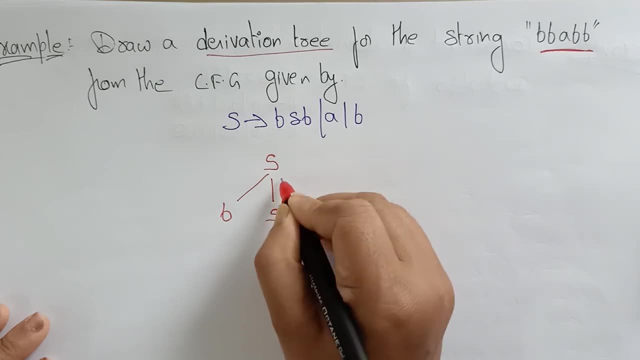 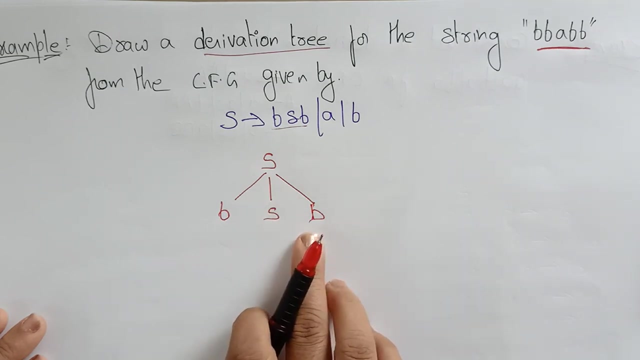 So here the start symbol is S, So starts with the S, So the S is can be substituted with B S B. Okay, The first prediction: the S is replaced with the B S B, So here B is already. it's a terminal. 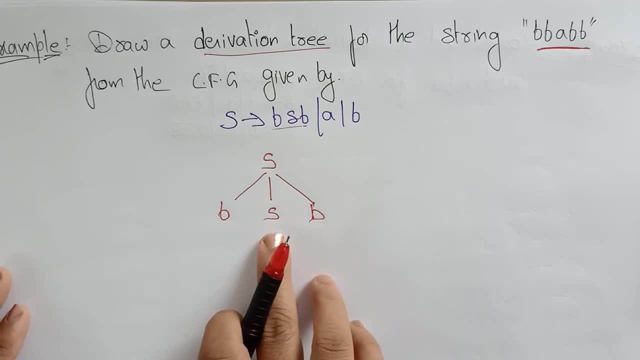 So don't touch it. Next, coming to the non-terminal. So here the S can be replaced with the A. So if I replace the S with A I'll get the string like B S B. So here the S can be replaced with the A. So if I replace the S with A I'll get the string like B S B. 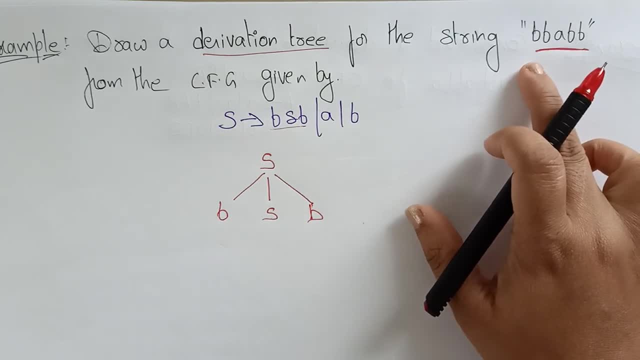 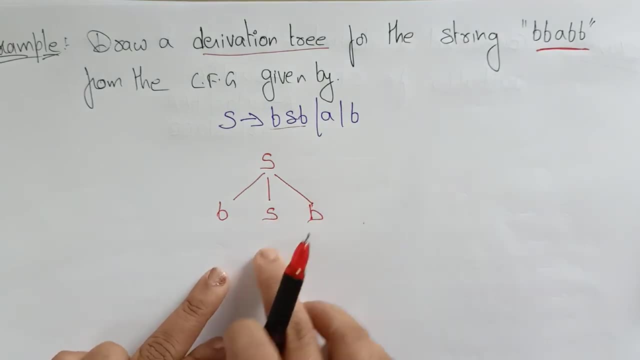 B, A, B. But according to our question, the input string that we need to derive in the derivation tree is a, B, B, A. So next I want to get the B. Suppose I substitute in place of S the B production. 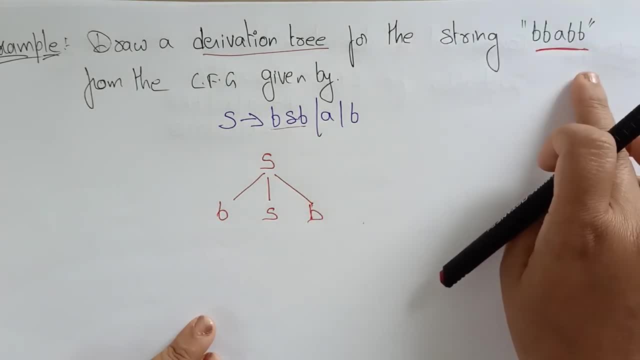 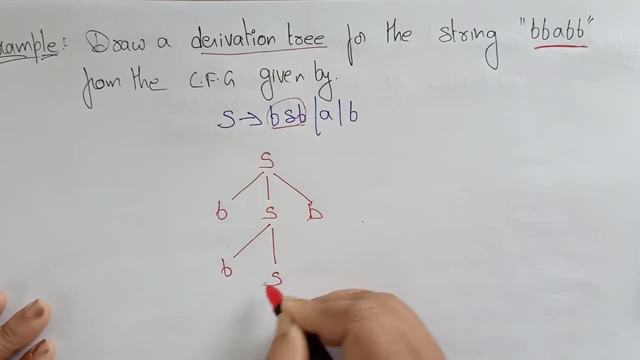 I'll get B B B, But here I want B A B B. So then what I had to do? Again, in place of S, substitute B S B. Okay, So now I got two B's. 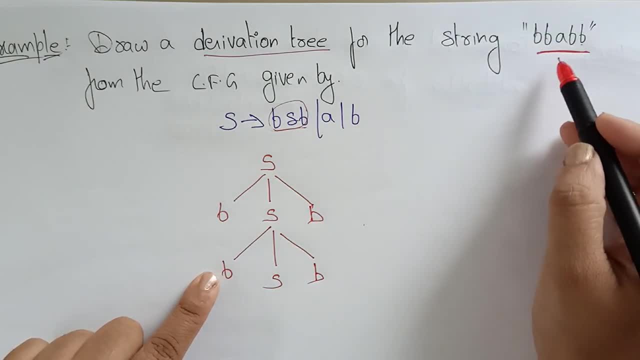 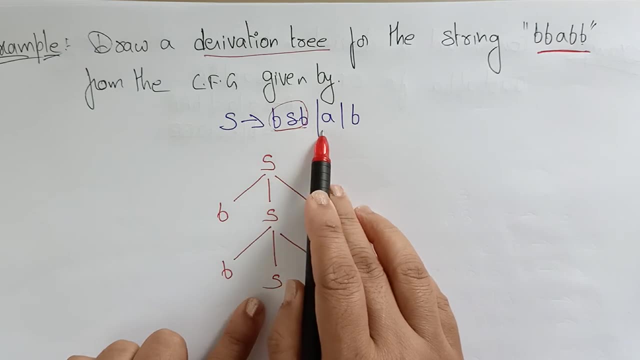 And here also two B's. So B, B, two B's are there, And what is the remaining string, that symbol that I need to get? That is the A. So in place of S you can substitute A, So then you'll get according. 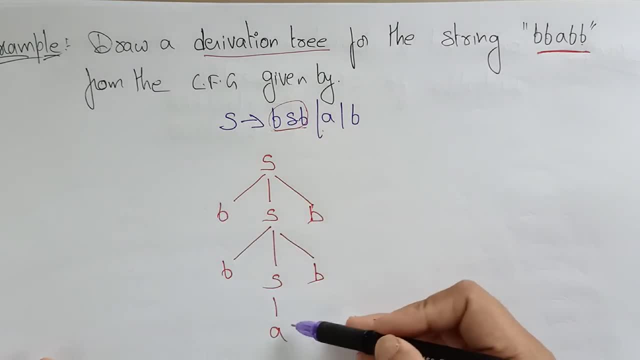 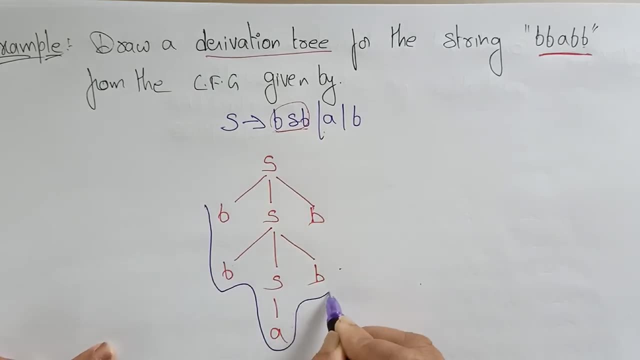 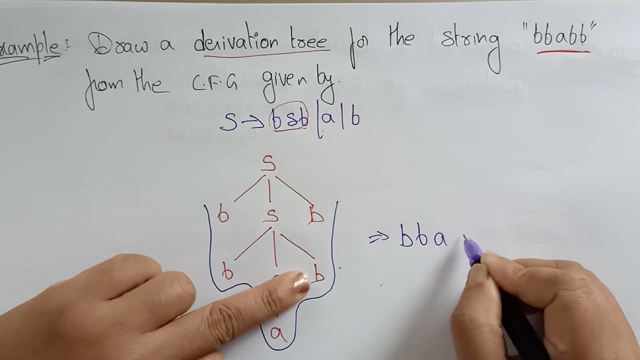 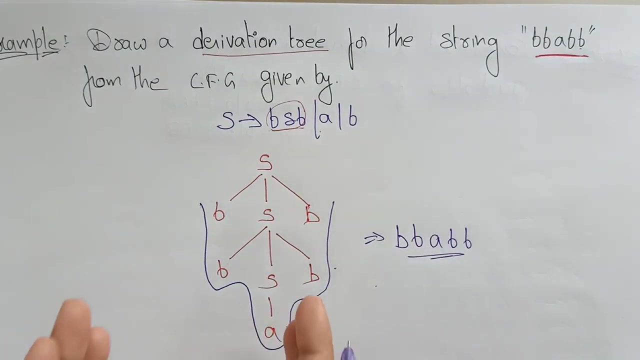 to our properties. the leaf nodes is always terminal nodes. The derivation is read from left to right, So starts with the left, and read from left to right, So what starts with the left- B, B, A, B B. So this is a string, what we need to get. So this string, it can be represented. 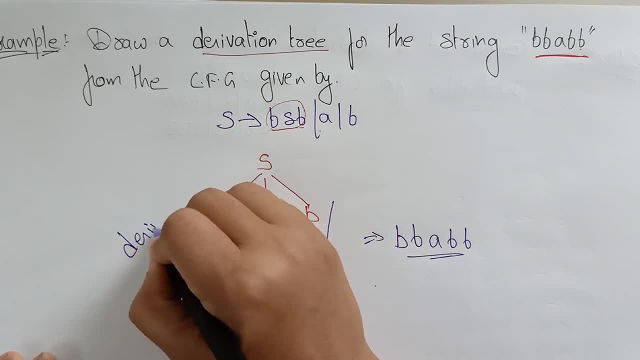 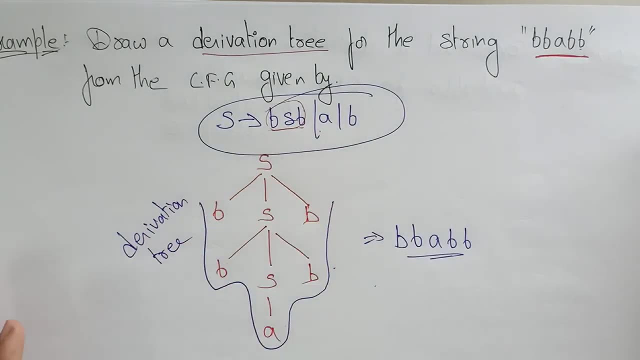 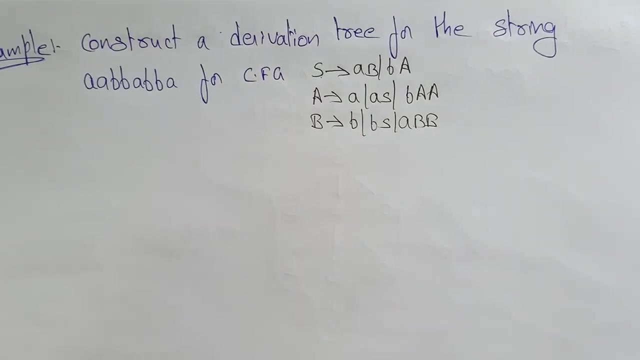 in the derivation tree. So this is a derivation tree In the form of a derivation tree, that is, a parse tree, by using this context-free grammars, that is, production rules. So let me take another example Here- construct a derivation tree for the string given. So this time I'm taking 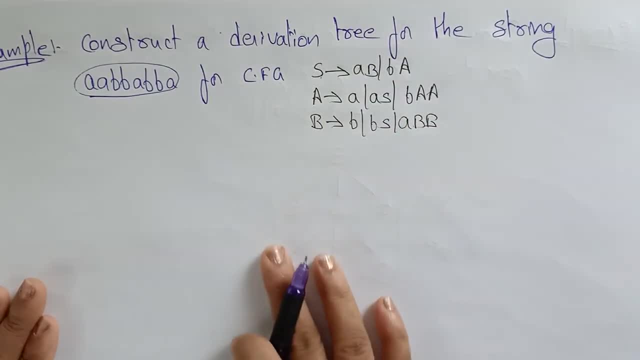 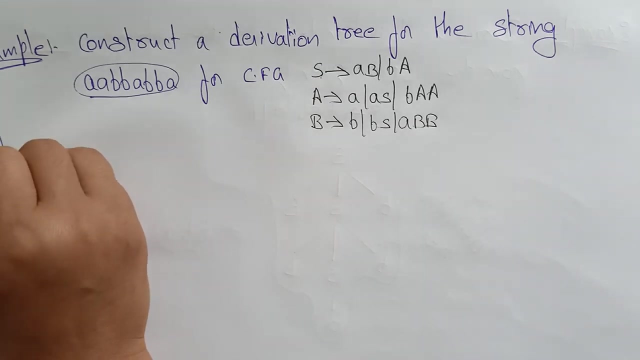 a big string for the context-free grammar. So here, before going to apply the derivation rule, derivation tree directly by taking the properties of the parse tree first, I need to derive the string by using the leftmost derivation. Okay, Leftmost derivation. So. 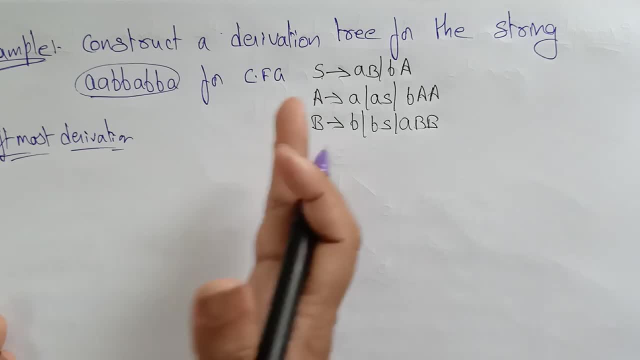 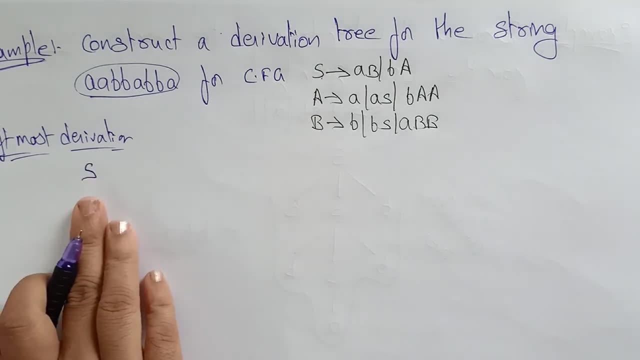 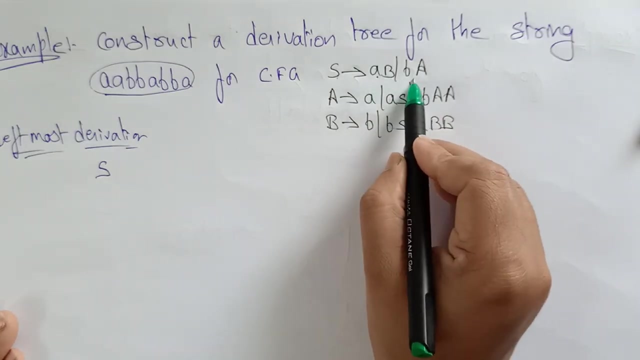 the leftmost derivation. with the help of this leftmost derivation I will construct the parse tree How Let's see here. So derivation should start always starts with the start symbol, S. Okay, So I started with S. So the S can be substituted with A, B or B A, But first this is the leftmost. 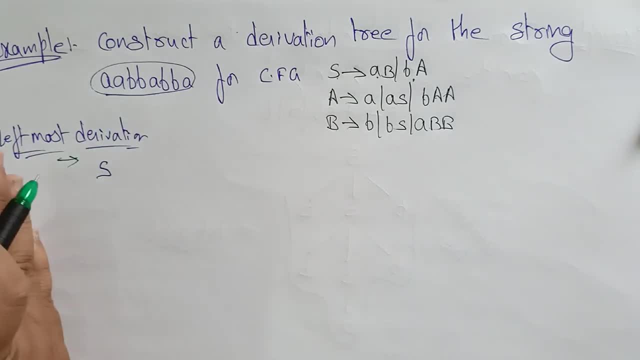 derivation means I want to read the non-terminals from left to right. So the first symbol in the string is A, So I need to substitute A, B, Okay. So in place of S, I substitute A, B, Okay. 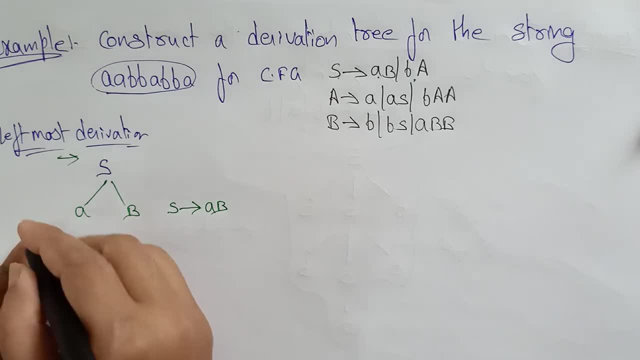 So I'm writing the rules. So now come to left to right. So this is the leftmost derivation: left to right. So here this is already a terminal, So no need to change. Now coming to the non-terminal B. So in place of B, which production I need to take? Either B or BS. 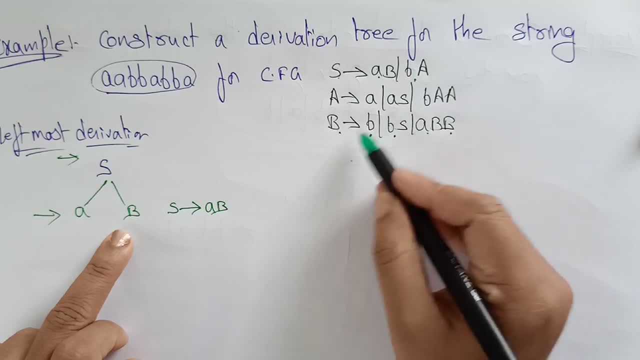 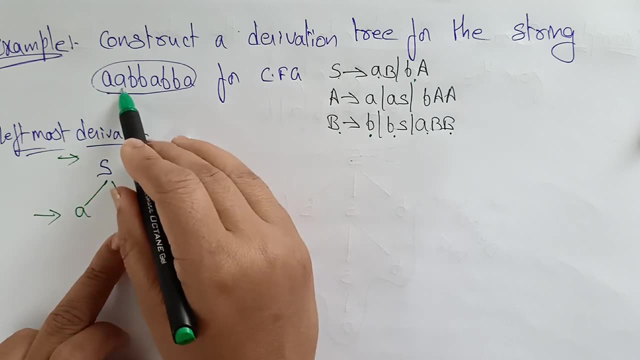 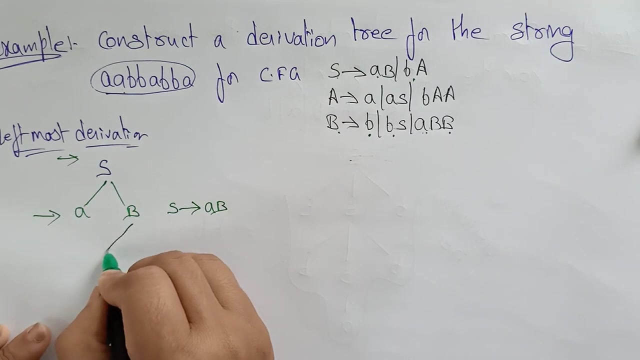 or ABB. So if you get a confusion, which production rule I need to take? means you just go to the string. So the next string is starting with means. after A, the next letter is symbol is A. So here A is in this third production. So let's take substitute in place of A. It's. 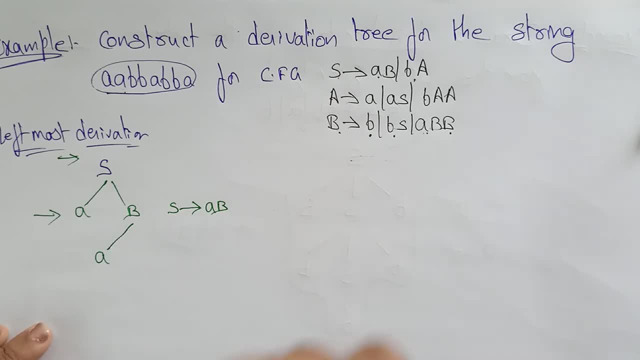 A: Sorry, I'm writing first, let me leftmost derivation. Okay, So in place of B I'm taking ABB. Substitute ABB. Later I'll draw that tree. Okay, So in place of B I substitute. 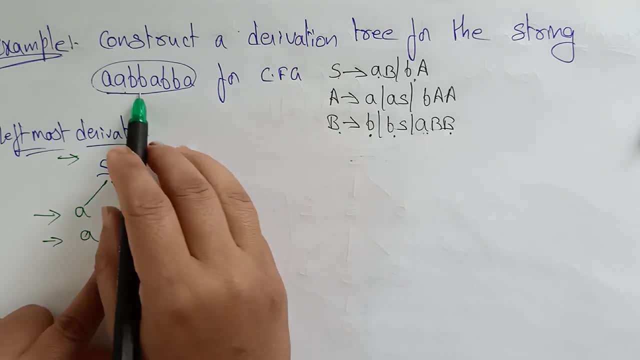 ABB. Okay, So I got two A's, So next I want to get the symbol B. So read the letters from left to right: So this is a non-terminal, this is a terminal and this is terminal. So the next non-terminal. 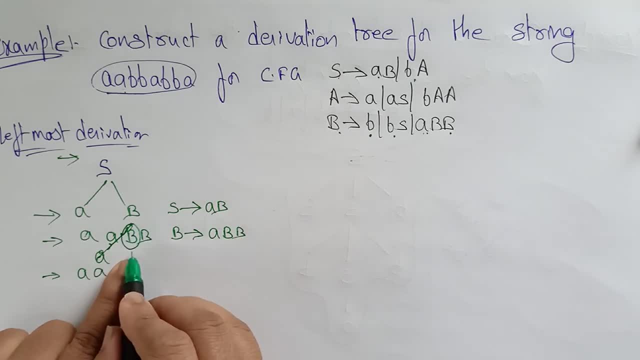 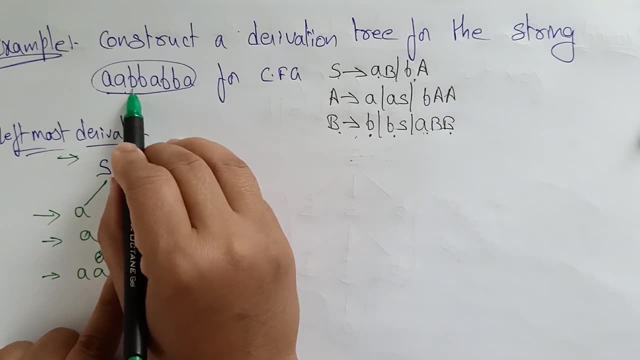 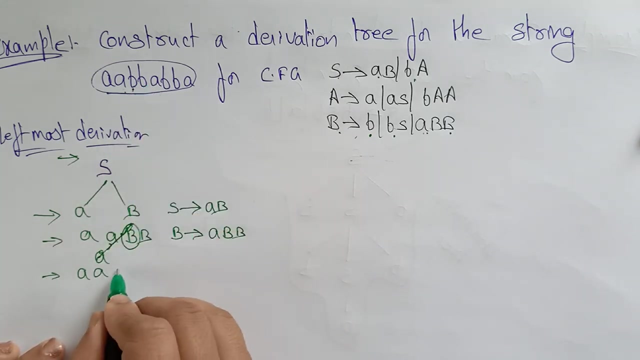 there are two B's, are there? First, you need to take the first B, So substitute a production in place of first B. So which production I need to take? This time I want to get B, Okay, So in place of B, I'm taking. 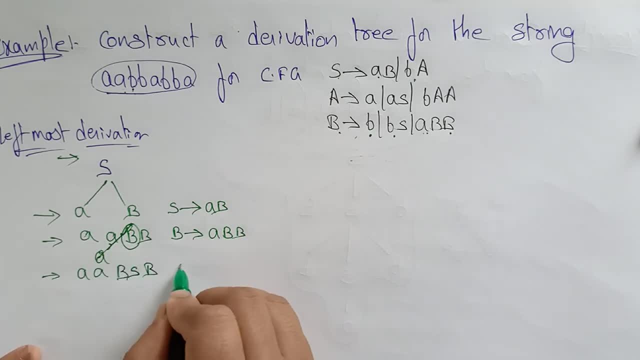 B S, B. So in place of B, I'm substituting B S. Now A next, what is the next non-terminal that is present here? So let me, this is small b. Okay, This is small b. Sorry, B S So. 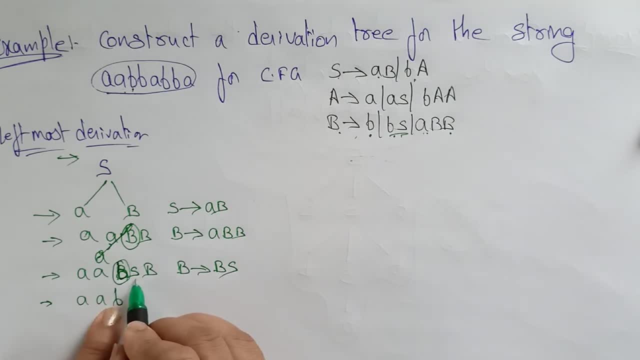 ABB is over. AAB is over. Next, S is there In place of S? which production I need to take? A, B or B A? Okay, So, in place of S, which production I need to take? A, B or B A? So, in place of S. 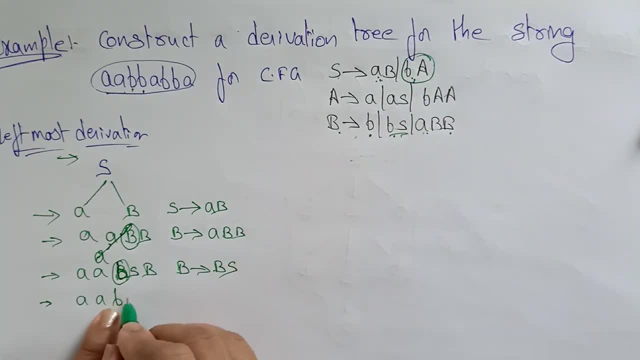 this string contains the next letter: is a, B, So I had to take BA. Okay, So in place of S, I'm substituting BA, B. So in place of S, substitute BA. Then next, what is the next non-terminal? A is terminal. A is terminal. B is terminal B is terminal. Now this A: 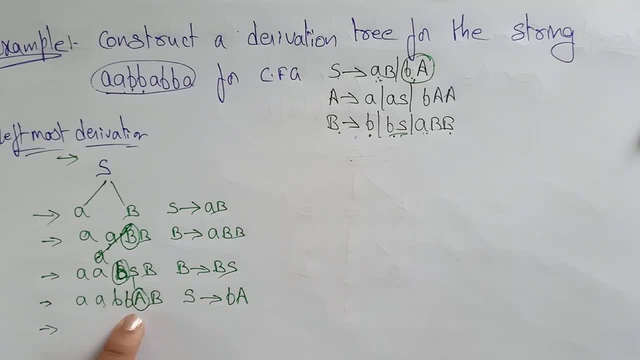 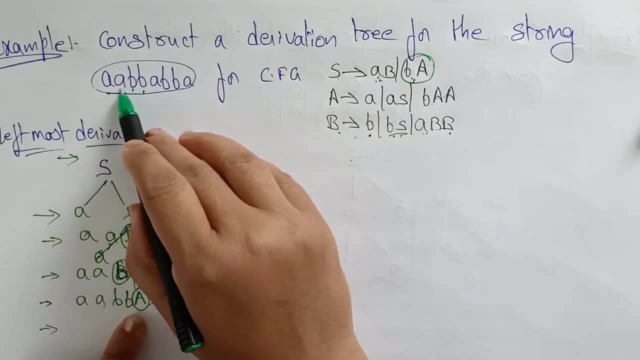 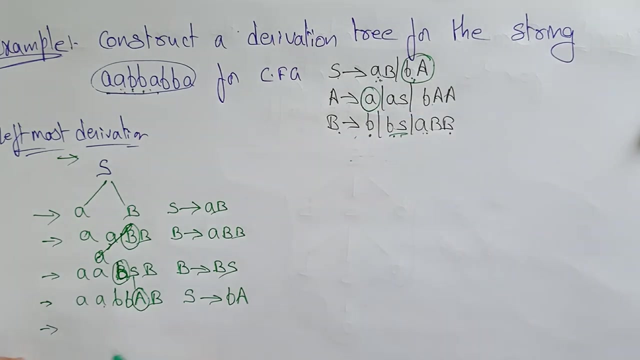 is a non-terminal So I'm scanning from left to right. Okay, Coming to the A productions, So which production I need to take. So check here. A is already visited. A is already. get B B over. Next A I need to get. So here in the A, I'll take this production. A, A, B, B, A, B. So 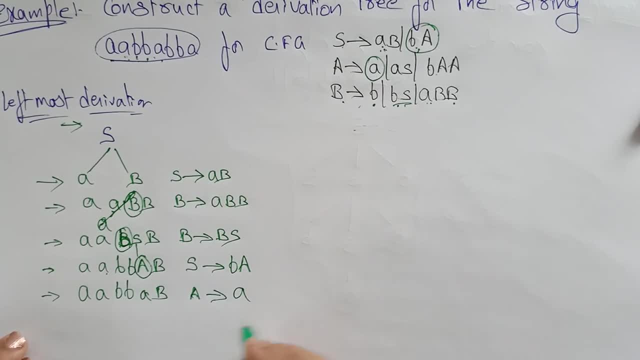 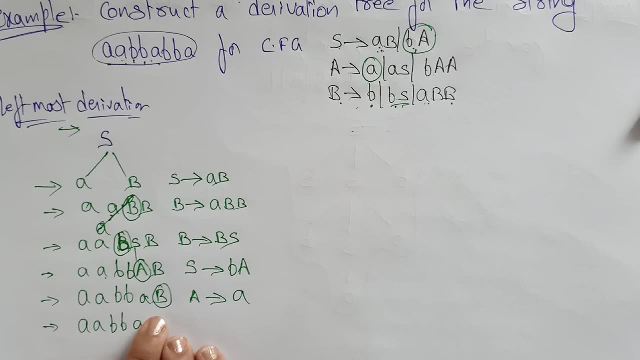 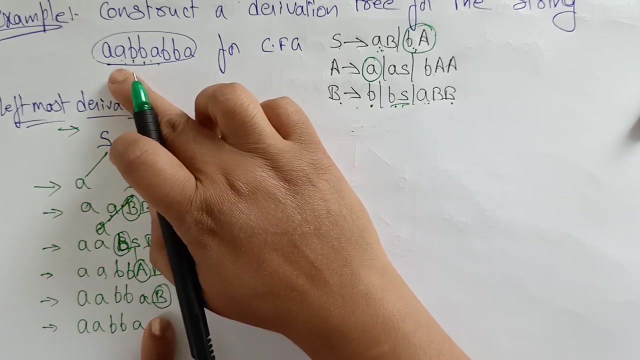 A is substituted with small a. Now coming to this: B, A, A, B, B. these are all the terminals and the remaining one, non-terminal, is a, B. So in place of B, which production? I have to take? Either B, BS or ABB. Okay, So see the string: A is over, A is over, B is over. 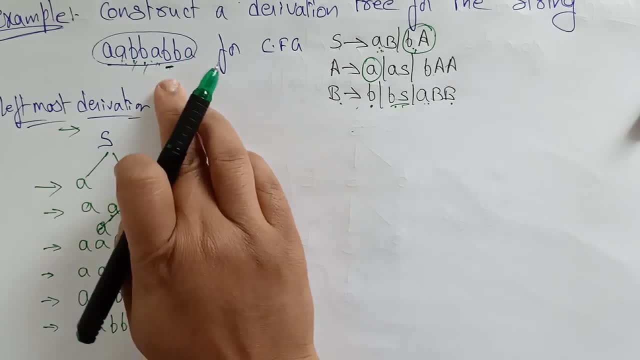 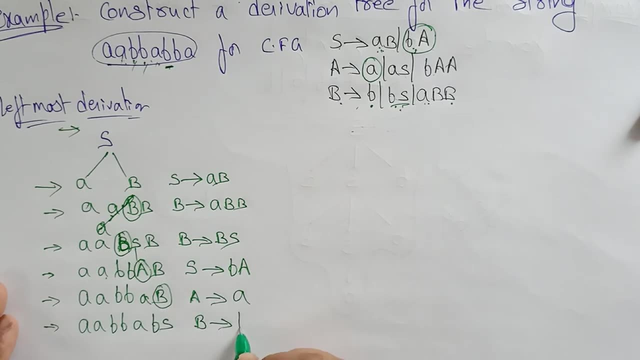 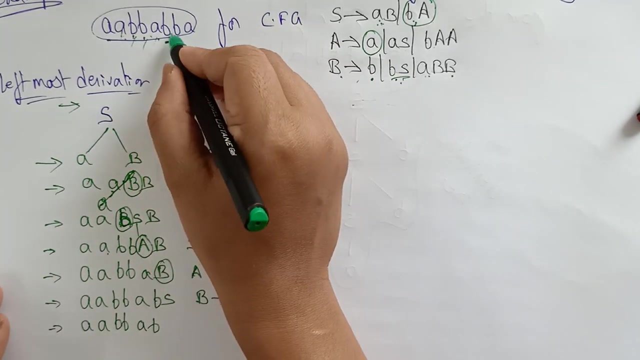 and A is also over, So next terminal is B, So I need to take BS In place of B. I need to take BS Next, A, A, B, B, A, B, up to here it is over Again: BA. So in place of 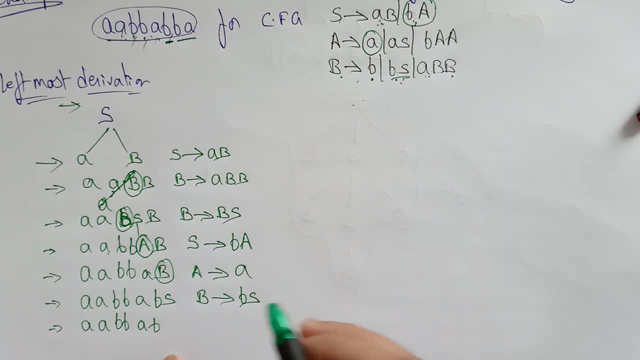 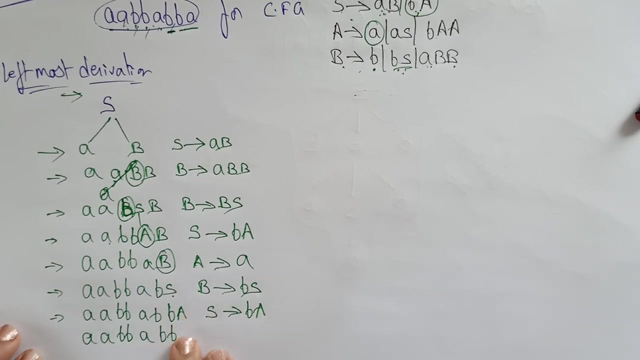 B, again, I'll substitute. So here. sorry, S is there, So S I need to take BA. So in place of S, take BA A, A, B, B, A, B B. So in place of A, just substitute A, So you'll. 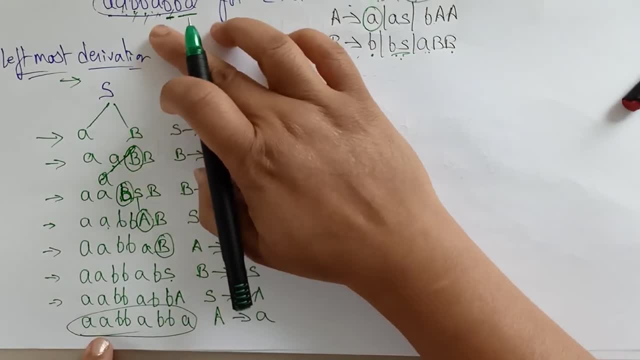 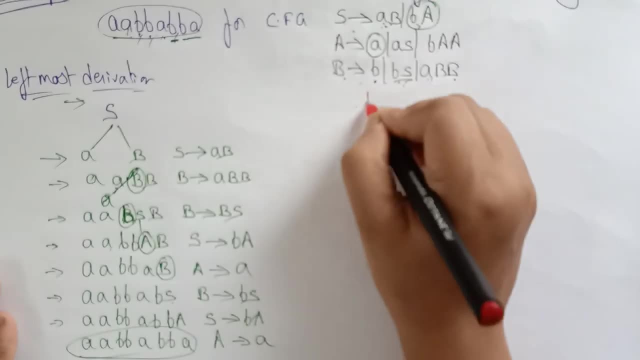 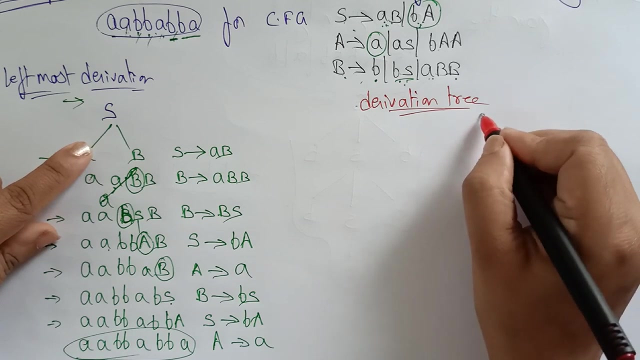 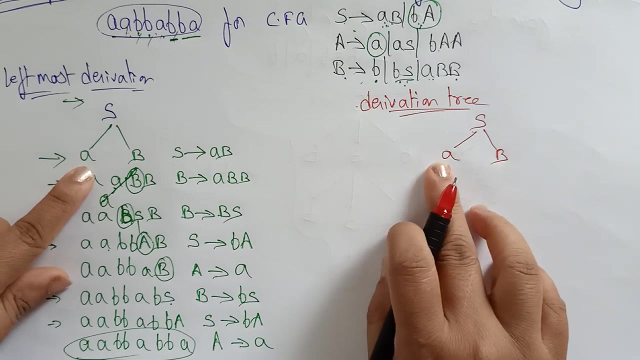 get the string that you pass: A, A, B, B, A, B, B, A. Okay, Now construct the derivation tree. So by seeing this leftmost derivation you can construct the derivation tree. So starts with the S, So S is substituted with A, B. Okay, So A is already. it's a terminal. 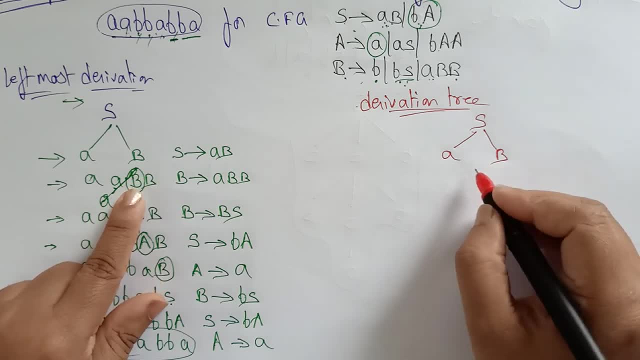 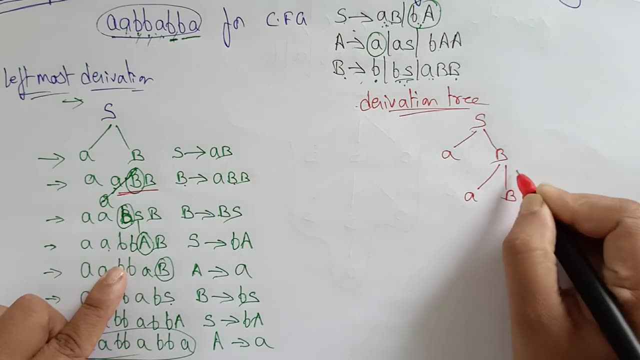 So go for the B. So in place of B, I write: I have written what I have written. In place of B, I substituted A, B, B. Okay. So coming to here, In place of B, I substituted BS. 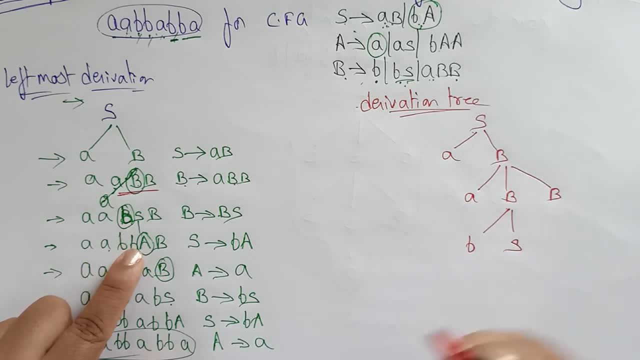 In place of B I substituted BS. So first come to here. So in place of B I substituted BS. So B is a terminal. So in place of S I substituted. in place of S I substituted BA BA. So in place of A, I. 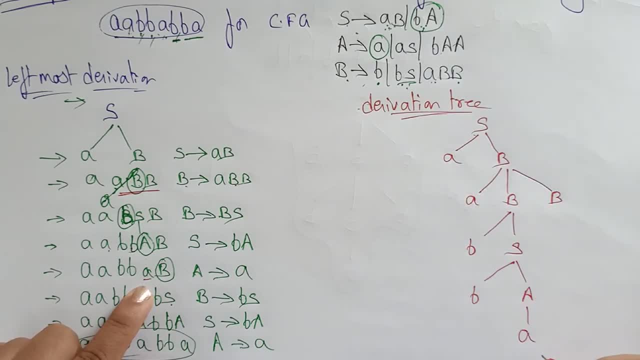 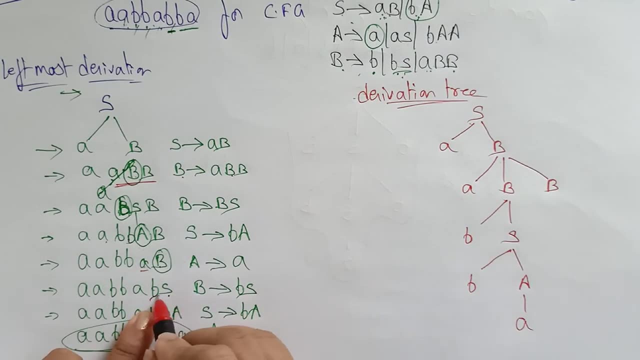 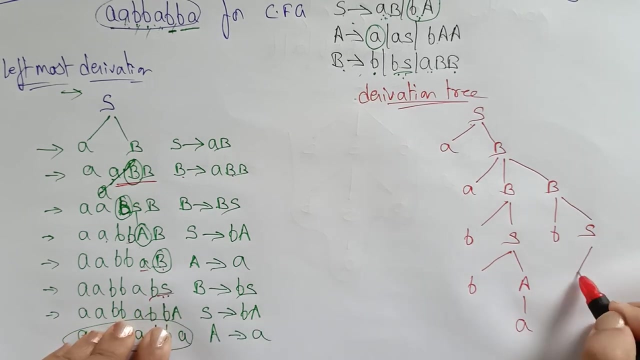 substituted A. So these are all the terminals Now coming to the B. Okay, So now, here in place of B, I substituted BS. In place of B, I substituted BS. Okay, So now, here in place of B, I substituted BS. In place of S, I substituted BA. In place of A, I substituted 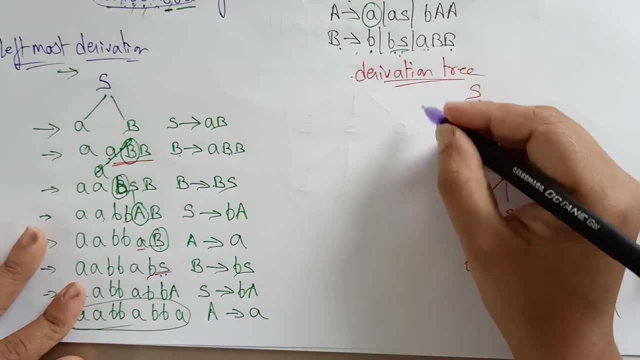 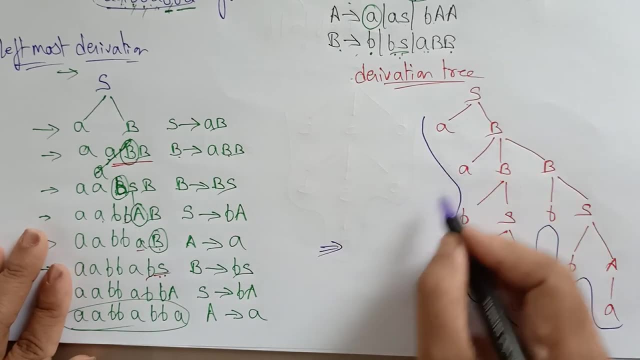 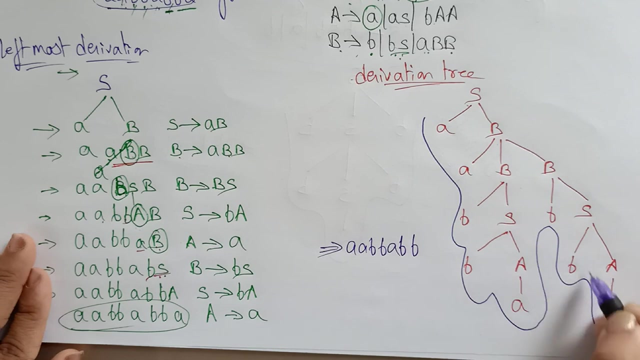 A. So now check. You had to scan from left to right. So what are the terminals? A, A, B, B, again A, B, B and finally A. So it's both the same. So in place of B I substituted: 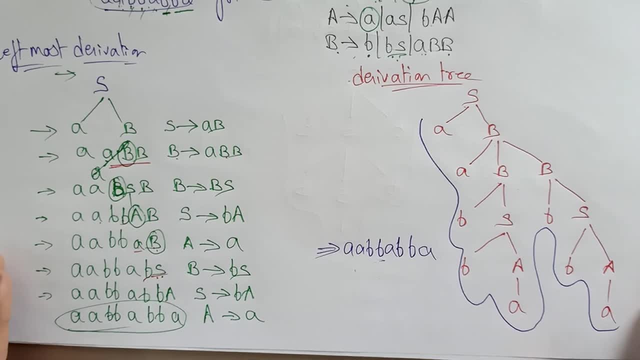 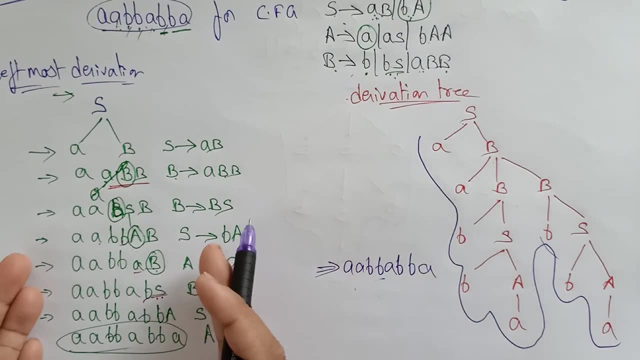 BS. Okay, So the strings are the same. Yes, So this is how you need to construct a derivation tree for the given string. So, if you want, you can directly construct the derivation tree, or else you can take the leftmost derivation or rightmost derivation. By seeing this, what? 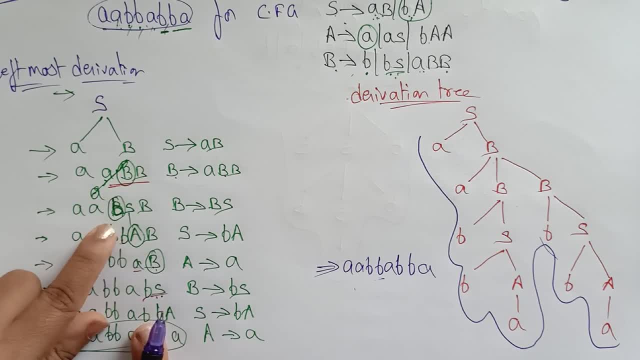 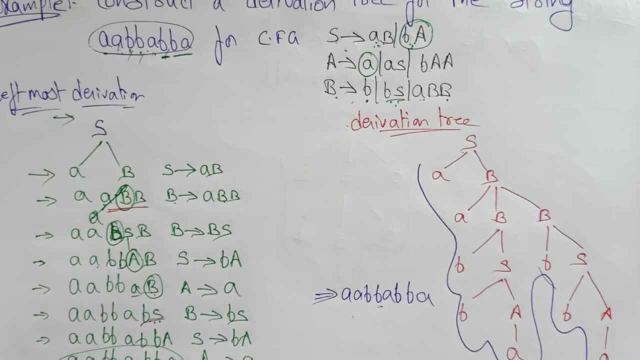 element that you substituted, what non-terminal is substituted with the production, So that in that way you can construct the derivation tree. So I'll talk one more example.